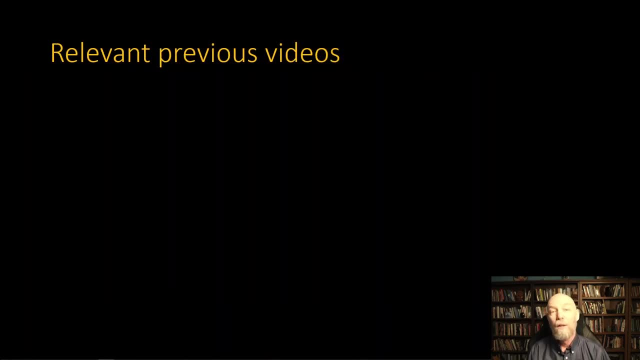 so that you can answer basic questions in applied settings. In the previous videos that I've done, there are several that you will need to be familiar with and you'll need to understand the information in them to be able to work with what I present here. There's a video on the. 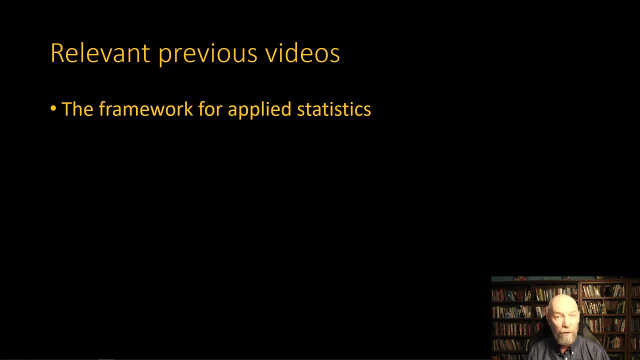 framework for applied statistics. so you understand what I'm trying to do and what I'm not trying to do. in these videos There's an introduction to the free statistical software package that I'm using. It doesn't have all the bells and whistles and some of the great features that paid statistical 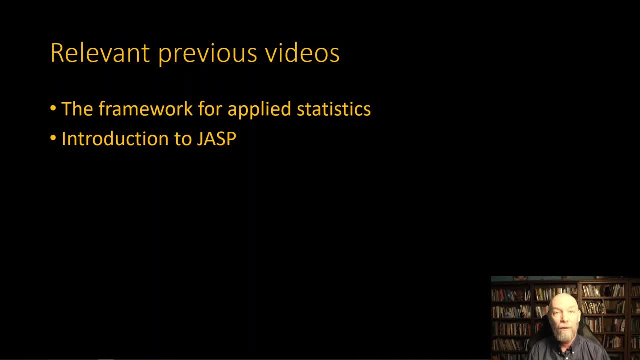 programs have, but it is something that a low budget circumstance can use to answer statistical questions. There's a video on shape, strength and significance, which will help you understand how unbiased statistical programs work and how to use them effectively. If you have any questions, 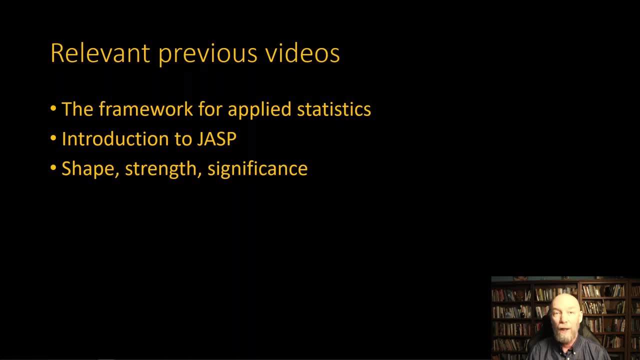 I tend to make sense of statistical results so that you can answer questions. There's a video on central tendency and dispersion. There's a particularly important video for this, one on correlation and bivariate regression. that lays the groundwork And in fact we will refer back to. 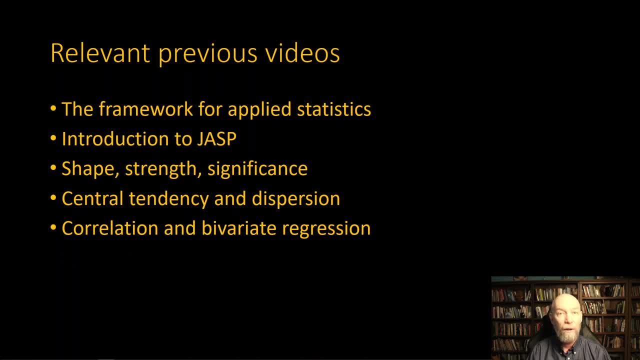 the material in that video, to be able to use the material in this video. And then there's a video on specification, which is a way of trying to make sense of how statistical controls affect our ability to answer questions. Now specification is a little bit more complicated. 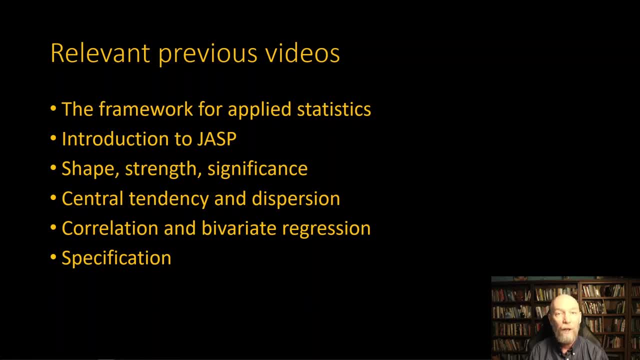 but specification as a term is used more commonly to just say how do variables relate to each other in a model, which variables belong in the model and where do they fit into the model relative to each other? But the way that we test specification of variable placement is through multivariate. 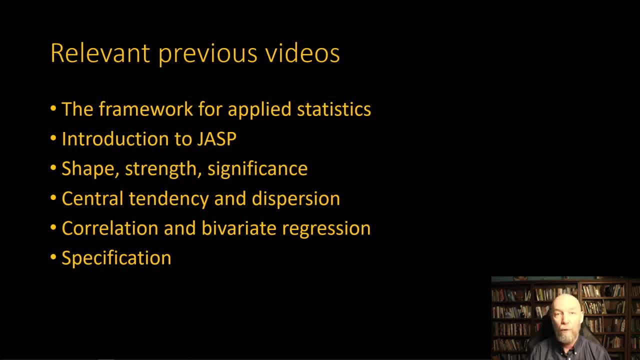 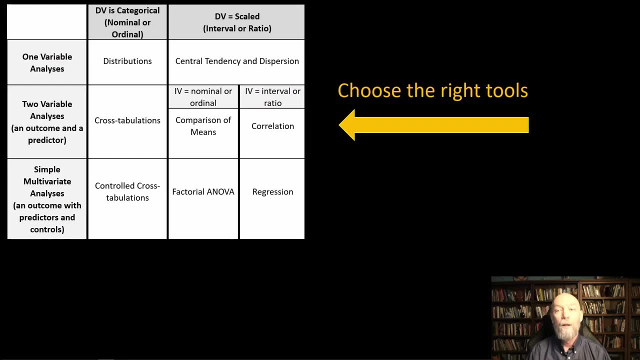 analyses. So, generally speaking, I'm using the term specification to refer to what we learn when we institute statistical controls in our analyses. The grid that I use for just choosing the statistical tools is an oversimplified grid that will guide you into choosing the tool that is. 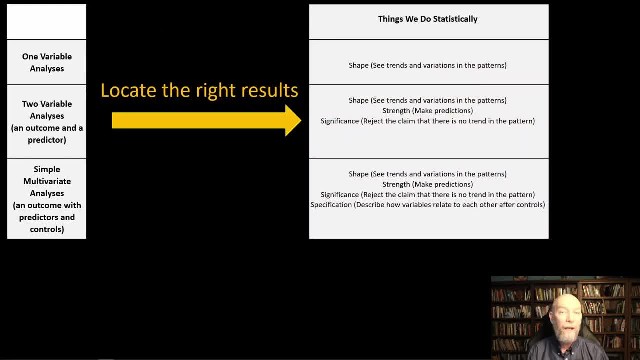 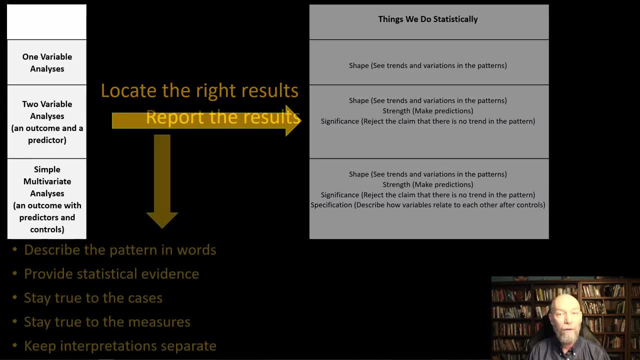 usually right most of the time for your setting. Then, once you've run those results from that tool, I suggest that there are a few things you need to be looking for to be able to answer the questions, And then I give five guidelines in this framework to try to introduce you to ways to avoid making 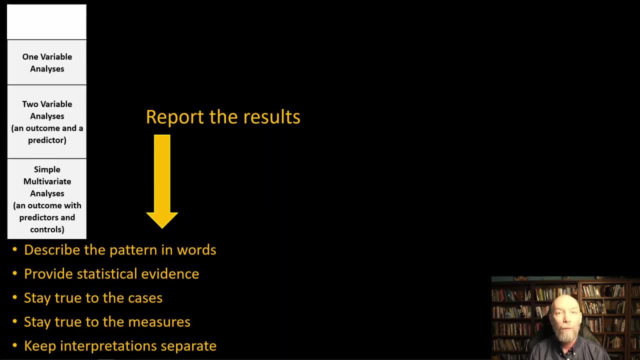 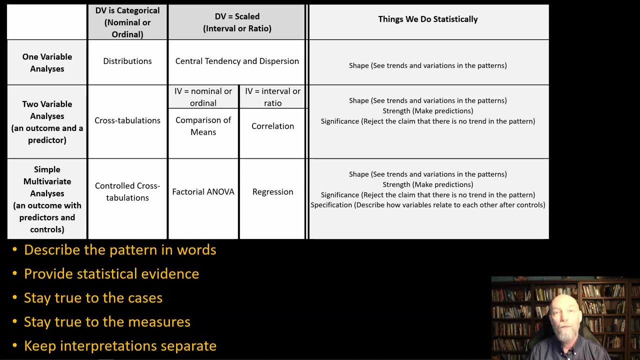 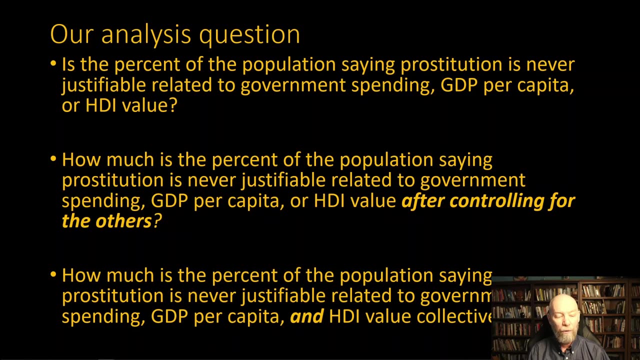 mistakes and still answer the real question when you present or write up your results. The overall grid, then, is meant for a more simplified approach rather than a simplified setting, but lays a good foundation for any advanced statistical work you might do later. I'm going to start with these analyses questions. I'm going to start with. 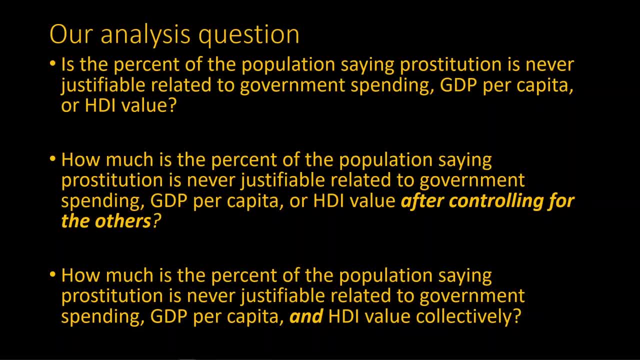 is the percent of the population saying prostitution is never justifiable related to government spending, GDP per capita or human development index value? Then, how much is the percent of the population saying prostitution is never justifiable related to government spending, GDP per capita or HDI? 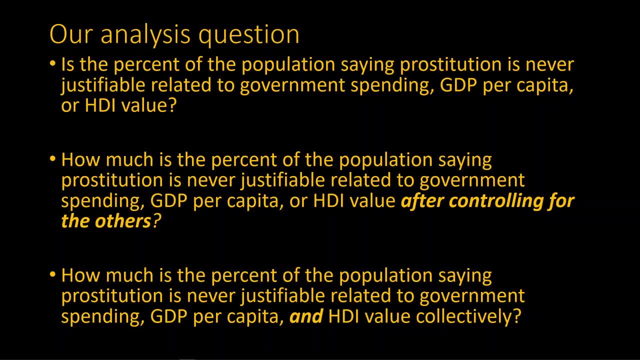 After we've controlled for the other independent variables. And third, how much is the percent of the population saying prostitution is never justifiable related to government spending, GDP per capita and HDI collectively? The first one is discussed in the correlation video. I won't unpack it here. 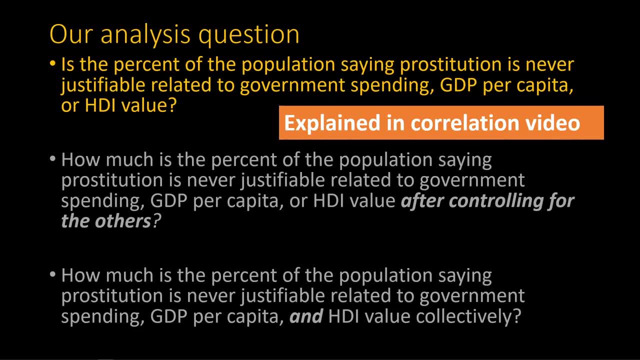 but you will have needed to answer that question before you can go on to answer the rest. The second question that asks how important is each independent variable after controlling for the effects of the other independent variables is an example of a net effects kind of multivariate. 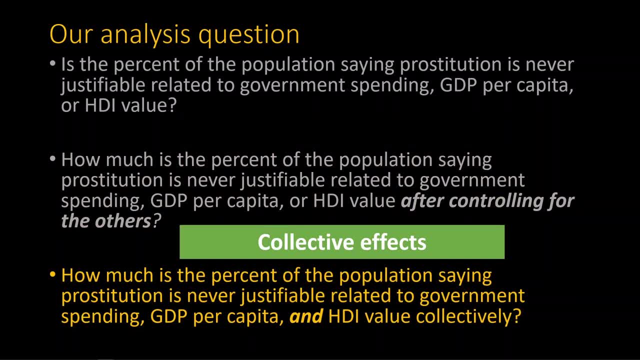 analysis. And the third question which asks: how much explanation do we get of the percent of the population holding this view? when we collectively look at the effects of all of these independent variables together, this is an example of a collective effect multivariate analysis. 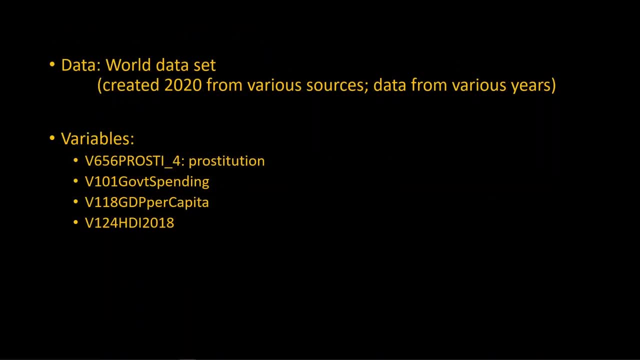 So the data that I'm going to use is going to be the world data set that we've been working with throughout this series of videos. The world data set is basically meant to introduce you to countries of the world in quantitative ways and get you thinking about using cases that. 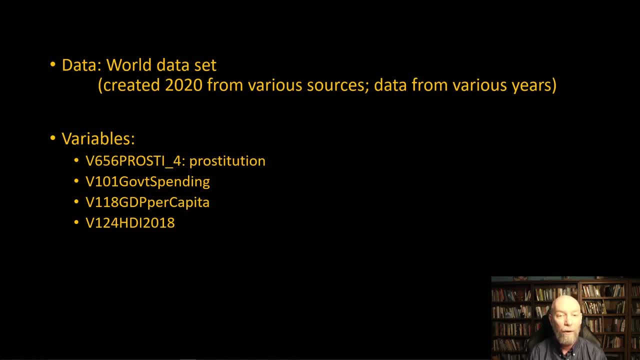 are different than just individuals, which most of us see more intuitively. The variables I'm going to work with, all of which have been used in previous videos. look at the fourth wave that was done in a series of countries about when is prostitution justifiable. 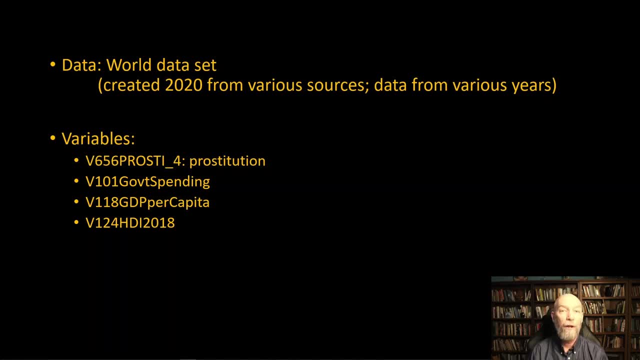 and for each country we have a number that says the percent of the population, that says it's never justifiable. We have a measure on government spending that's been discussed in previous videos: a measure of gross domestic product per capita and a measure of the human development index. 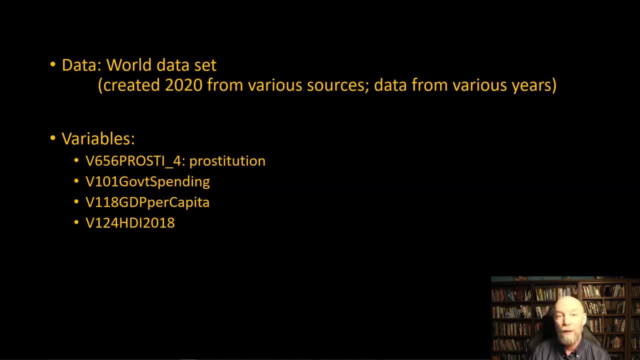 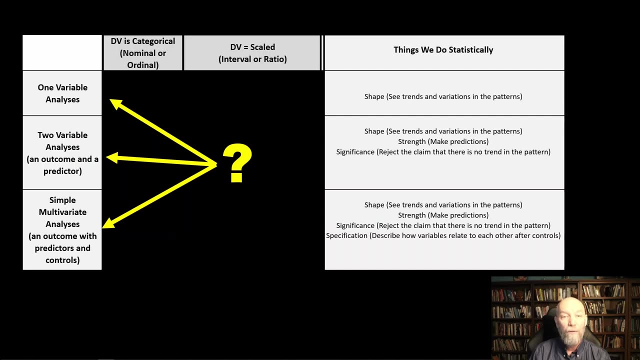 values from 2018.. All of these variables have been explained and unpacked in previous videos. In the choosing grid, we have to first decide if we're doing one variable analysis. we're just going to take each of these variables by itself and look at the results in it. 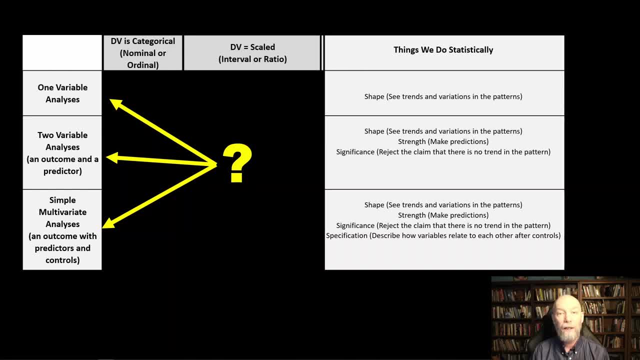 or if we're doing two variable analyses, where we want to basically take an independent and connect it in pattern analysis to the dependent variable and see if they're related. or if we're doing multivariate analysis, where we have independence and a dependent but we also statistically control for the effects of some variables while looking at the relationship. 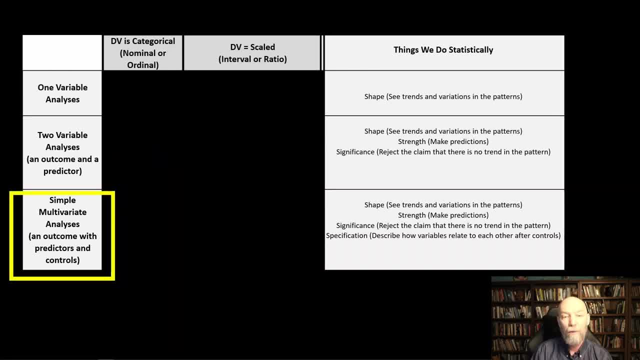 In this case, we're doing a simple multivariate analysis, so any statistical tool we use is going to be in this row. The dependent variable is the percent of the population believing that prostitution is never justifiable. This is a scaled variable, and so we end up in this column. 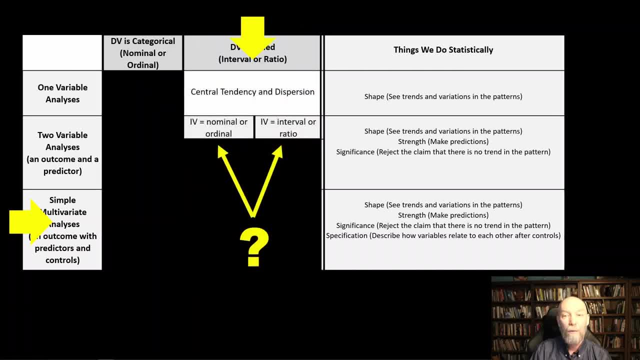 As we move down the column, we find that we have to decide if the independent variable is categorical or if the independent variables are interval or ratio. All of our independent variables in this example are interval or ratio, so we're going to use the independent variable. 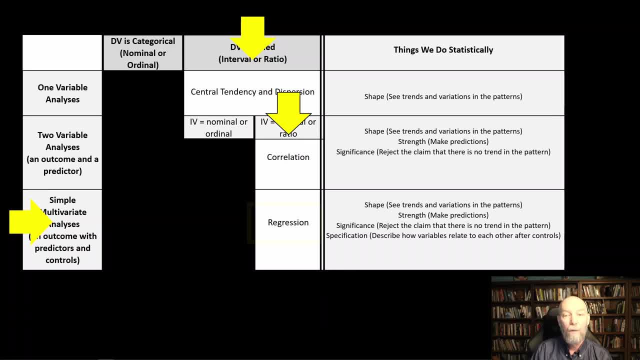 The independent variables in this example are interval or ratio. so we end up in this column: When we grid that out, we end up with multivariate regression, and so we need to look to answer questions at the shape, the strength, the significance and the specification. 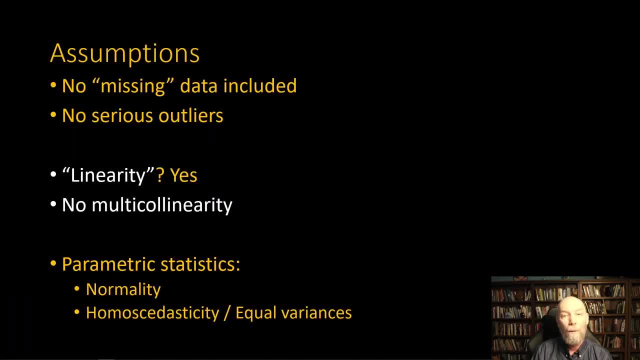 the way I've described what those are in previous videos, to be able to answer our questions Now, there are some assumptions that happen when we're looking at multivariate regression. First, we assume that none of the cases have non-valid or quote-unquote. 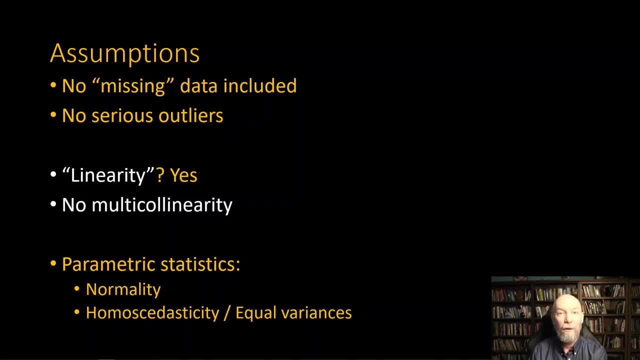 non-variable data, But we assume that this is a zero-value regression, so we need to look at the various variables in this way. I've cleaned up this data set so that any data values that may have stood for this country doesn't have a value for this variable, or this is a number that 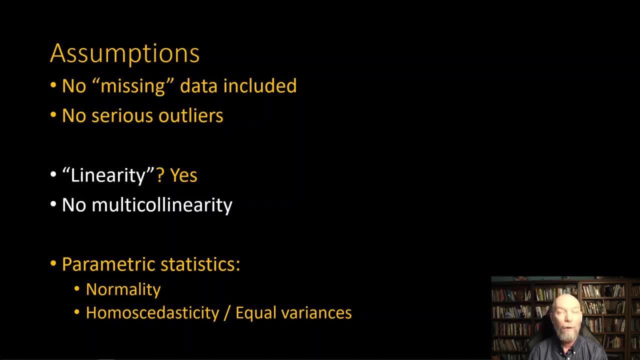 indicates something unusual for the country. that isn't really about what the variable measures. all of those have been removed. It assumes there are no serious outliers. In the last video I showed you an example of a bivariate outlier in the correlation scatterplot that was shown and so 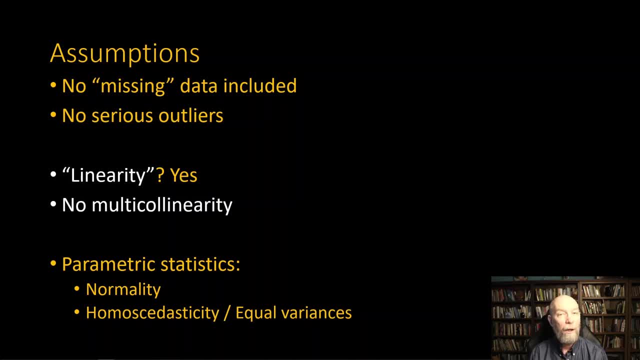 kinds of outliers. There is an assumption of linearity, but I put it in quotes now because we have more than two variables related. It's beyond the scope of this video to explain it. but when we add two or three or four independent variables to the model and we run the mathematics, 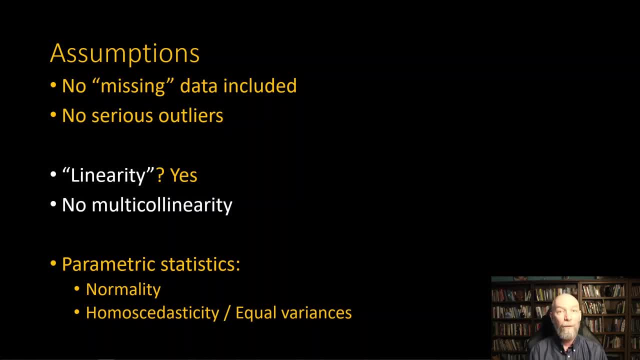 we're not just talking about a straight line. That's what we could have if we have an x-axis variable and a y-axis variable, and then we have a straight line, best fitting line as our prediction model. That's what we did in bivariate correlation. but in this circumstance, if we have 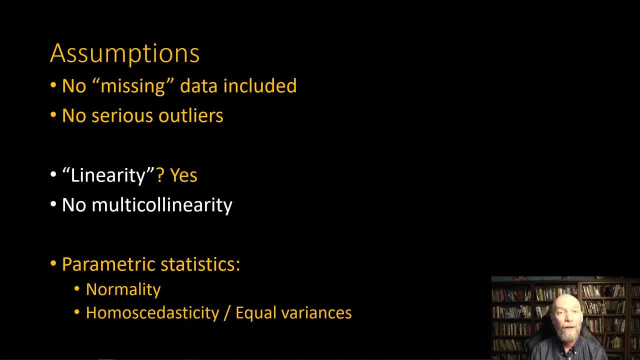 two or three or four independent variables, or however many we have, we actually end up with a multi-dimensional, best fitting project, and that is still assuming a certain kind of flat surface. but it begins to boggle the mind to be able to conceptualize a three or four or five-dimensional. 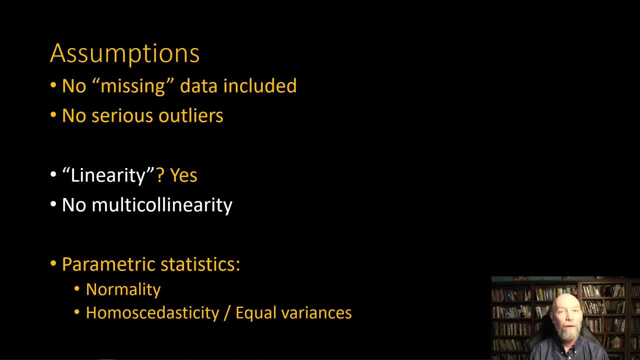 flat surface. So we're just going to say there is still an assumption of linearity, Curved relationships are not seen. but we're not going to try to unpack that any more than that. Now we have a new assumption here that there will be no multi-collinearity. 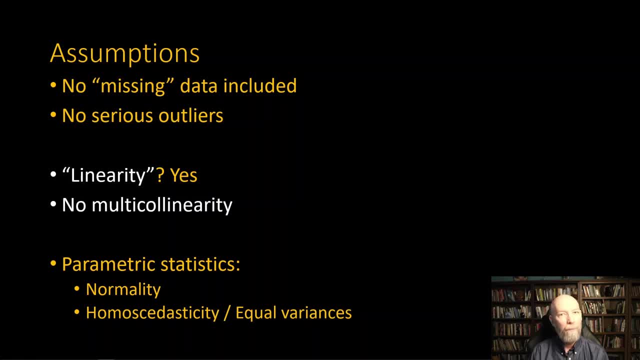 involved in the model. I'll explain that in a moment. but basically it's saying our independent variables cannot be strongly related to each other. This isn't to say that an independent variable cannot be strongly related to the dependent variable. That's fine, That's great. 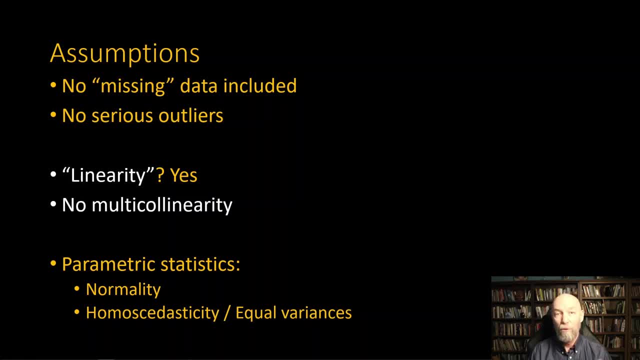 Don't worry. Don't worry about ever seeing an independent variable connected strongly mathematically to the dependent variable. but when independent variables are strongly related to each other, there's a problem using the mathematics of multivariate regression. These are parametric statistics. 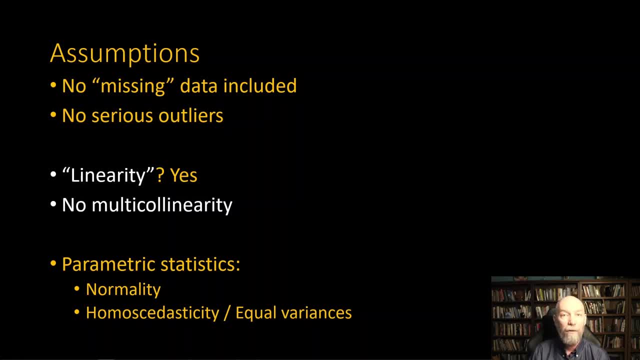 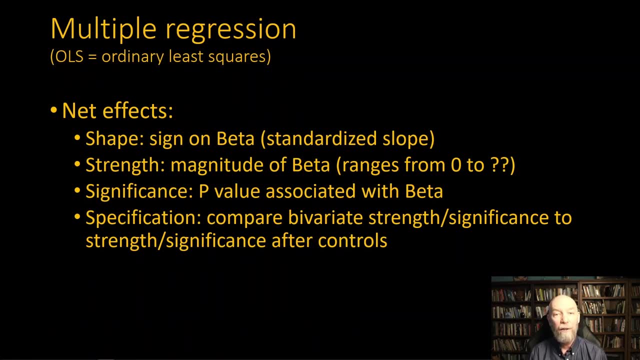 and so they assume normality and homoscedasticity, as has been discussed in previous videos. So multiple regression that we're using here is something called ordinary least squares regression. In the prior video I showed a best-fitting line and a scatter plot and I talked about how you measure all those distances between. 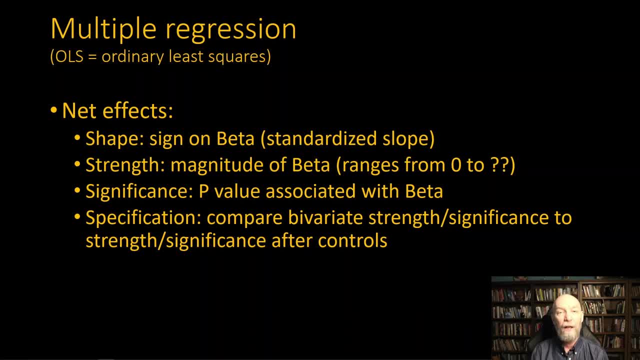 the actual case plottings and the prediction line and you add them all up. Well, what you really do is you take that distance, you square it and you add them all up, and that's called the ordinary least squares. You want a line or a prediction plane or a prediction three-dimensional. 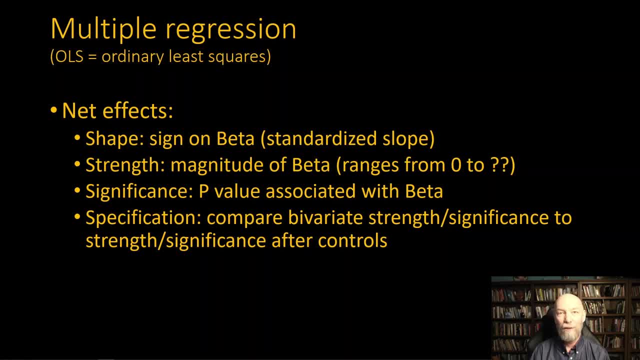 linear model. You want all of these prediction models to have the least error in correctly placing where the cases end up, And so ordinary- least squares, least squared deviations. Now, it's ordinary in the sense that you can have a variety of other versions of this that are beyond. 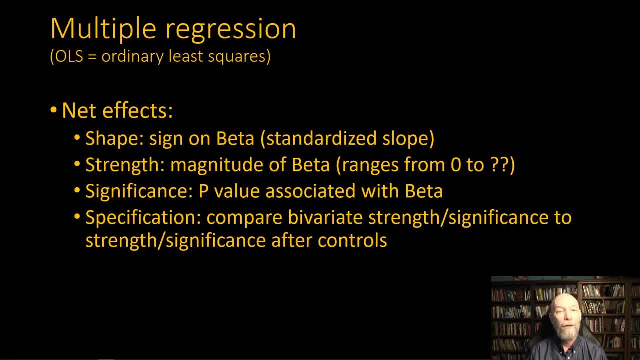 our scope here: Two-stage least squares, weighted least squares. So regression is a very robust and valuable tool and we're looking at the most commonly used version of it. Whenever somebody presents you with regression results with no other name, they don't call it logistic regression or 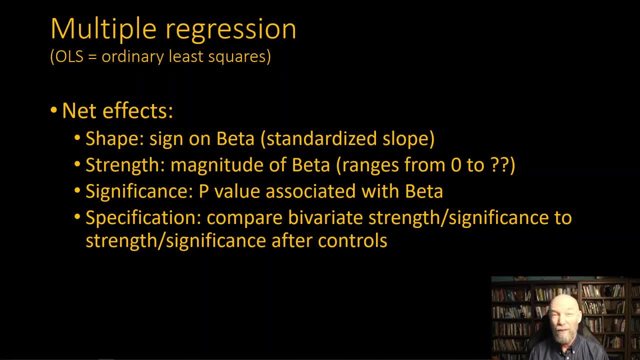 some other name. they just say: here are the regression results. it is almost always ordinary least squares linear regression, All right, so in the specification video I talked about how statistical controls can help us to do something called net effect analyses, something called collective effect analyses, something called interaction effect analyses. 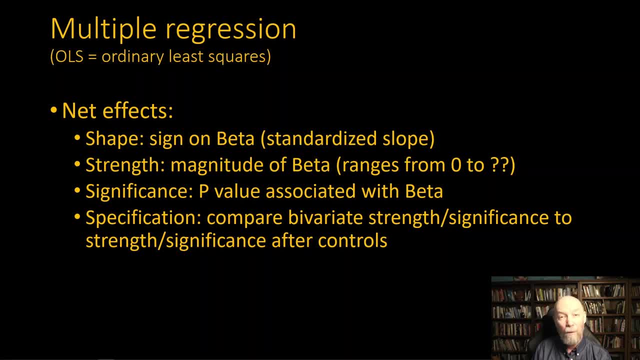 and can also help us to specify a causal model. Multiple regression does allow us to do net effect analyses, And so what we're going to look for when we look at some results is we're going to look for shape by looking at a direction of effect in the sign on what's called the beta And the beta. 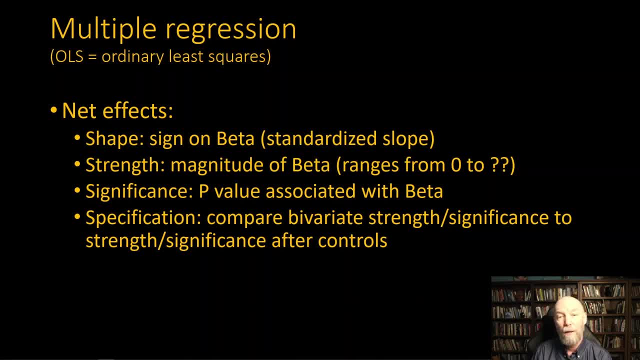 is the standardized slope That'll be unpacked here in a minute. The strength is found from the actual number, the value of beta Or the magnitude. It ranges from zero to some undefined upper limit and we'll explain that in a moment. But in essence, like we did with r, where we looked at the sign and said: is it a negative relationship or a positive relationship With beta, we look and we say it is a negative or a positive beta. And like r, where we looked at the magnitude and we said: is it closer to zero or closer to one? In this circumstance we're going to look at the beta and we're going to say: is it closer to zero or is it a bigger? 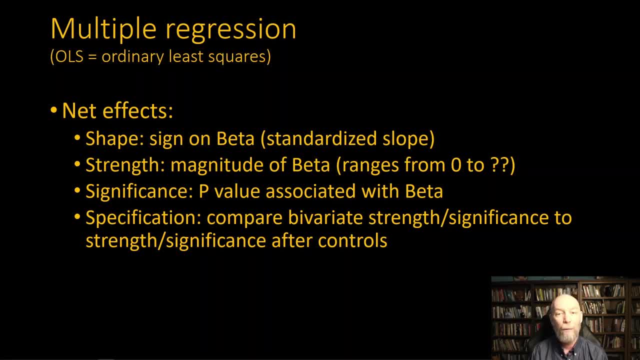 number as it moves away from zero, Because there's no defined upper limit In significance. we're going to use a p-value associated with beta and it works just like the p-values have always worked. It's telling us the probability that we would get the real-world results we did if, in fact, the null hypothesis was true in the real-world population data. So we're trying to find out a little test here, to find out if we can reject the null and say no, we really think something is probably going on in the population. 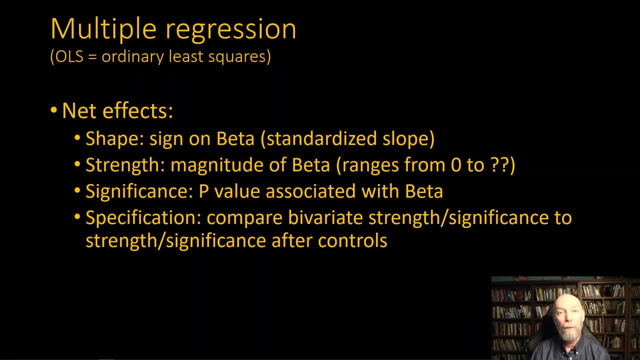 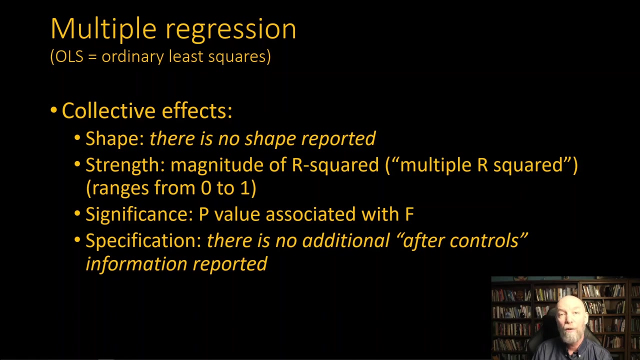 Because we don't think the null is true. The probabilities are against the null being true. And then, in terms of specification, what we're going to do here for most of this is we're going to compare the bivariate strength and significance to the strength and significance we find in the betas after controls. That's the net effect. Collective effects are also talked about in multiple regression, and this is the first tool in this video series that has had a collective effect measure. There is no shape. 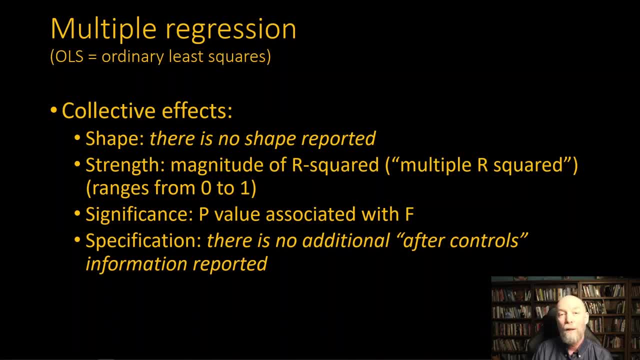 reported. I'll unpack that when we get to the example. But there is no way to talk about direction of effect because if we have two or three or four or five independent variables, some of them are causing the dependent values to go up, Some of them are causing the dependent values to go down, And so collectively what they're doing can't be described as up or down, except in a net sense, because we have to take all of them into account. So collective effects is just summing up how much effect overall is being explained. 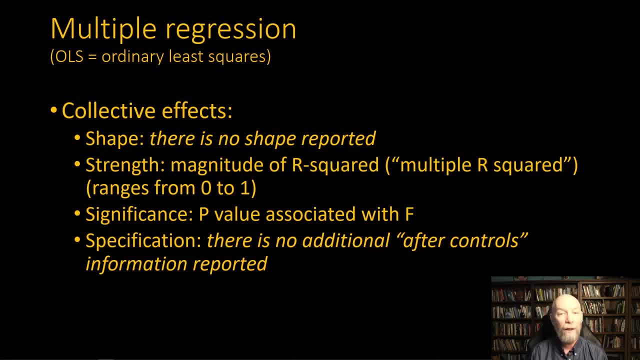 by this set of independent variables and we can't have a direction. So there's no shape reported in collective effects from multiple regression. Strength is reported by the magnitude, the actual value, the size of the number of a tool called R squared. Now it's capital, R it's the multiple correlation coefficient and then the multiple correlation coefficient is squared. thus multiple R squared. This ranges from zero to one, like so many tools we've looked at. So as you get closer to the end of the video series, we're going to talk about how to do that. 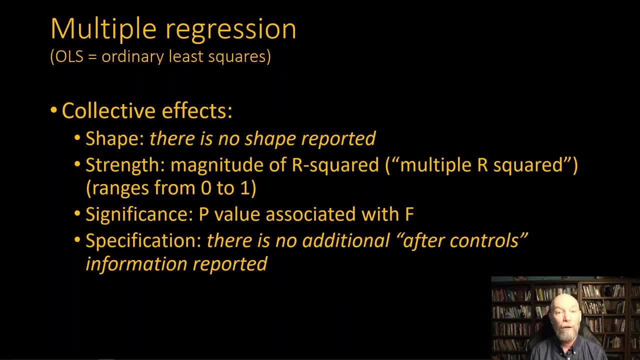 closer to zero, the collection of independent variables are explaining nothing. and as you get near one, the collection of independent variables are explaining all of the variation in the dependent variable. There's a significance, p a probability value, just like all p values. This: 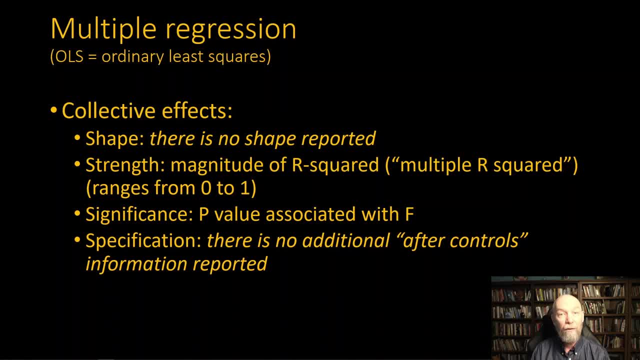 one comes from an f-test. It is another analysis of variance, just like what has been used in previous examples and other videos. There's a different mathematics of how we decide what pieces go into the f-ratio, but it's the same f-test and so there's a p value from that f-test. 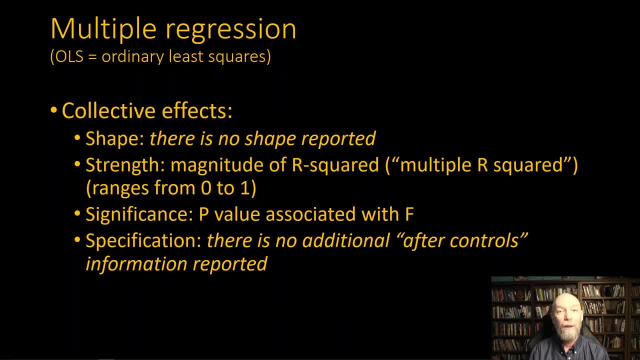 and it is the one that tells us the probability that we could get the real world multiple r squared. we have- if in fact multiple r squared was equal to zero in the population- the null hypothesis. And then there's specification: There's no additional after-controls information reported. 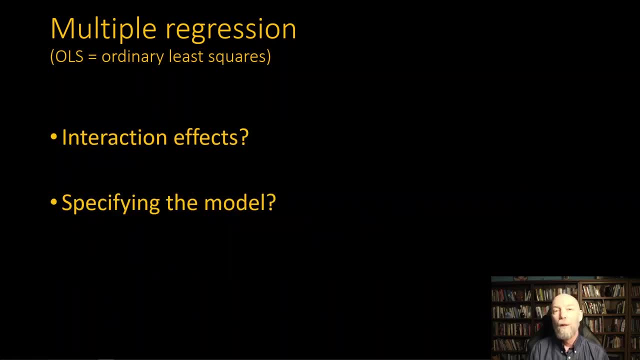 in collective effects. It is polyphonic possible with simple OLS regression to look at interaction effects, but it's beyond the scope of what I'm going to do here. But any basic stats book that talks about dummy variables, just go looking for one that talks about dummy variables and you'll find out how to put in categorical. 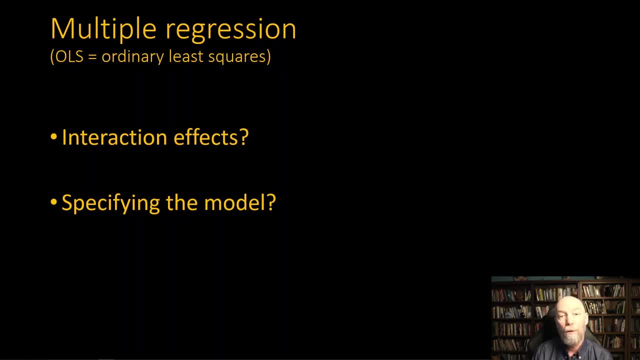 variables, But usually I use that as kind of the baseline. Once they start talking about that, they usually also talk about other things. Another thing that could be talked about is interaction effects and interaction effects of how two independent variables or any pair or three. 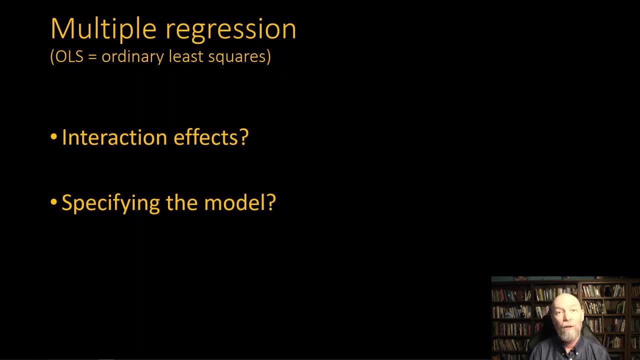 or four independent variables collectively interact and affect each other's effect on the dependent variable starts getting a little complicated. We won't look at interaction effects here, but it is possible in simple multivariate regression or just a little beyond simple multivariate regression, to look at interaction effects And in terms of specifying. 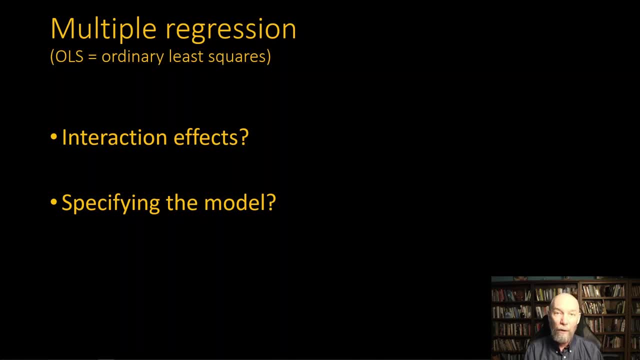 the causal model in terms of deciding which variables go where in the model and have arrows pointing at other variables. we're going to talk about that in a little bit. All of these results, particularly the net effects and interaction effects, help us to specify a model. 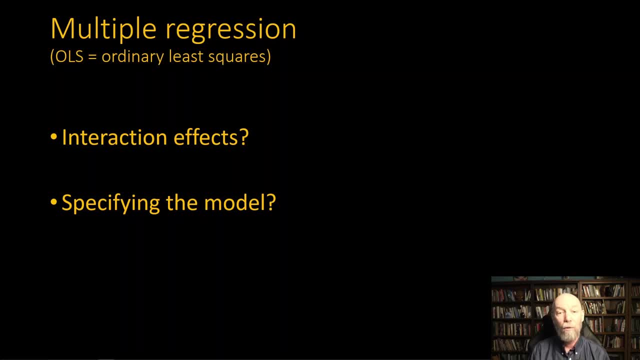 We're just not going to go that extra step in this video series to look at how we would interpret it, because it involves a conceptual step quite a bit beyond what we're doing with our basic applied statistical work here. So let's jump over to the analysis program and let's take a look at how we 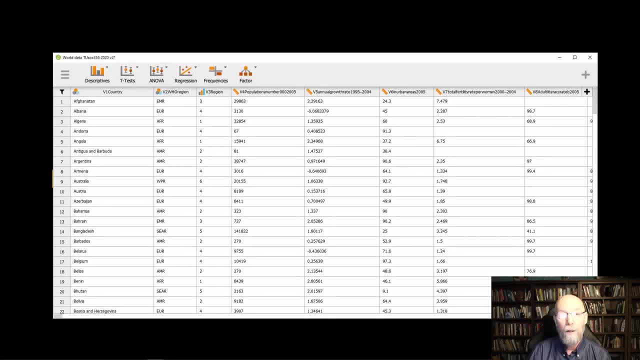 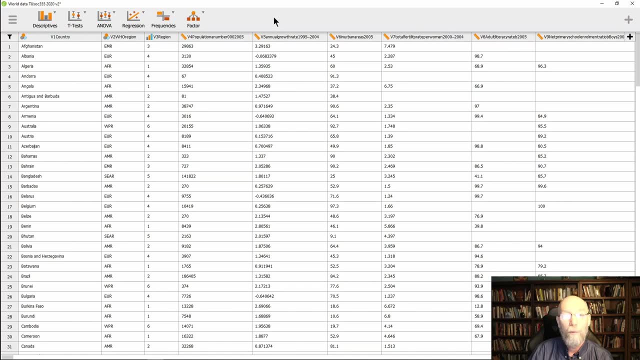 would do multivariate regression. I've already opened the analysis program and I'm going to go into the regression option here and I'm going to choose first correlation. Now, that's not our point here. We want to look at linear regression, but I'm going to start with correlation because we need to have 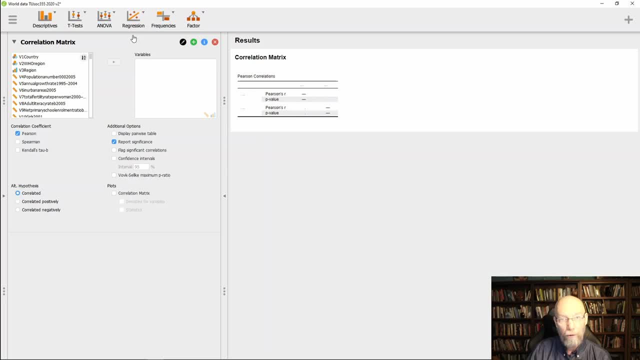 the results of the correlation matrix, to be able to use the results of the multivariate regression to make sense of what we've learned after statistical controls. Our dependent variable is the 656th variable in this data set that I've put together, so I'm going to put it first. 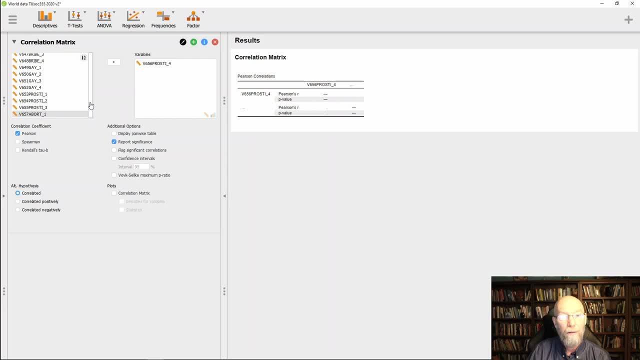 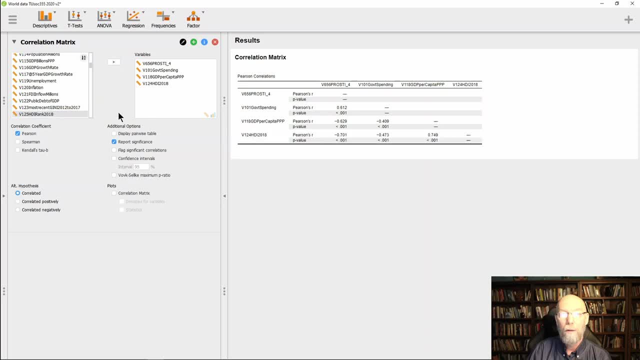 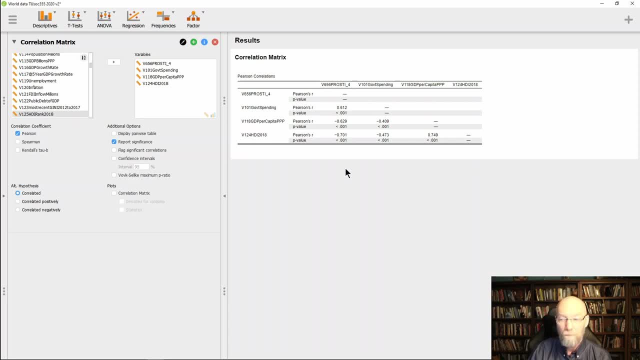 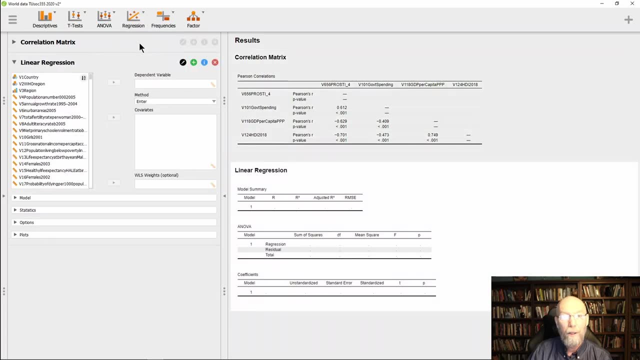 We're going to need that to be able to make sense of the multivariate. OK, let's set that aside. We'll come back and look at those results in a moment. Now what we want to do is we want to then go ahead and do linear regression. 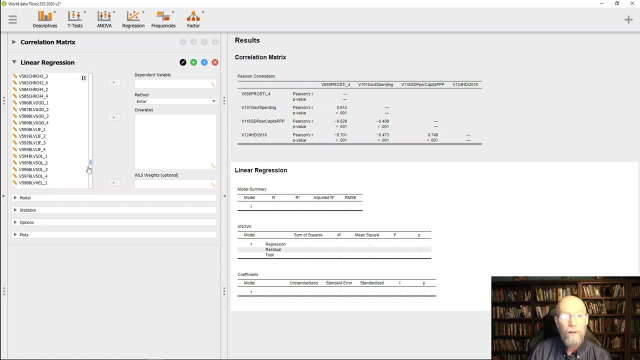 And again we want to choose the dependent variable as 656.. So now we're going to add the correlation matrix 56.. We're going to use the same enter method that was talked about in the previous video for bivariate regression. It's the most commonly used version of OLS regression. And then we're 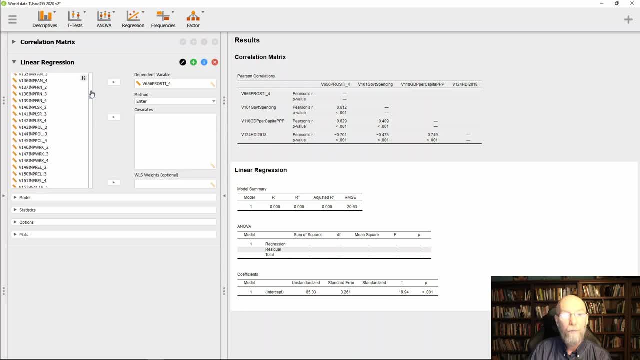 going to put in our independent variables, starting with 101, government spending, then 118 for the GDP per capita, and then the HDI value. Okay, now that's how you would run it. You don't really, with this particular tool, need to do anything more. You don't need to go in and 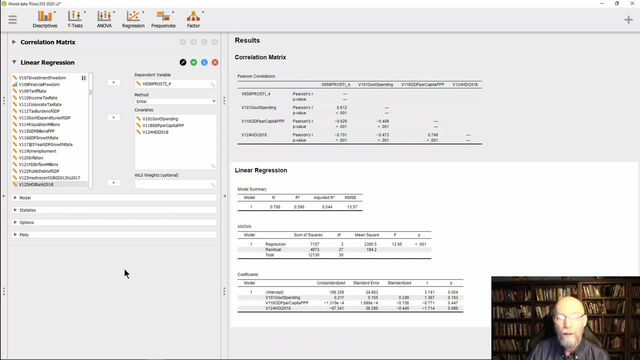 specify model or statistics or options or plots. You can basically work from what we have there on the screen. We're going to discuss the problem here. I'm going to unpack this as we look at the results in just a moment, But there's a 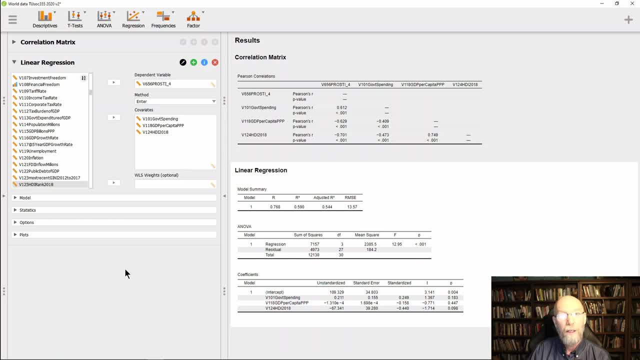 problem here. There's a violation of the multicollinearity assumption, And so we're going to have to remove a variable from our analysis. I'll explain why in a second. But basically, we need to take GDP per capita and we need to make it go away, And these are the results that we're going to. 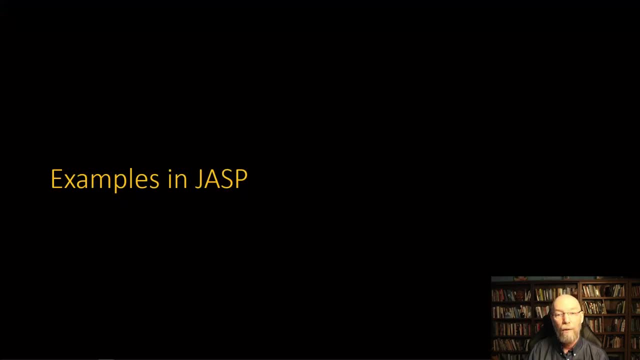 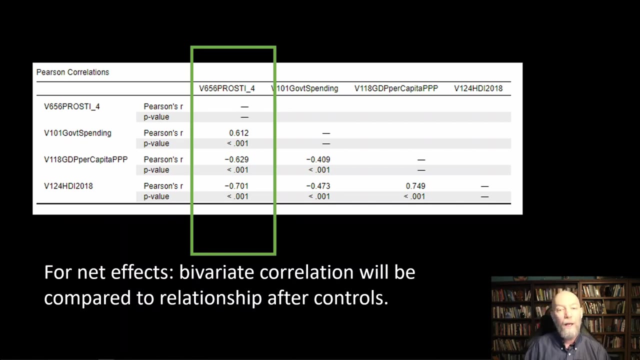 work with, But that's how you would actually run it in JASP. Okay, So here's the correlation matrix For the net effects. we're going to have to know what the bivariate correlations were. So we can see that prostitution view in the countries is related strongly to 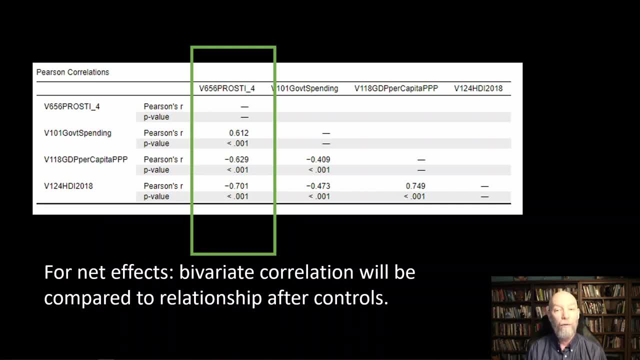 government spending in the countries with a correlation coefficient that's 0.6.. It's a positive relationship. Those countries that tend to spend more are countries that also tend to have a larger percent of the population. Now, we don't care now about the GDP per capita, because I've already removed it from the multivariate. 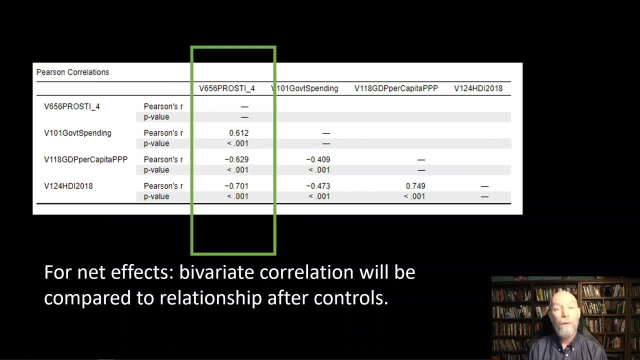 regression and I'll explain why in just a second. But we do care about the human development index value And that again is a strong 0.7, a very strong relationship between HDI value and view of prostitution. But now it's a negative effect. So now we see that as countries have higher, 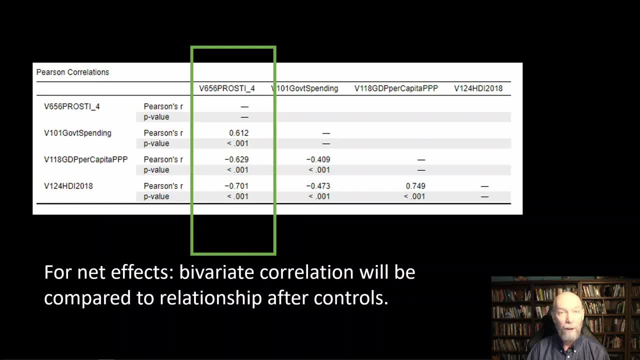 human development index values where the population has more education, higher average income, longer life expectancy. where that's true, there tends to be a lower percent. As HDI goes up, negative effect: prostitution goes down. The view of prostitution is never justifiable drops. 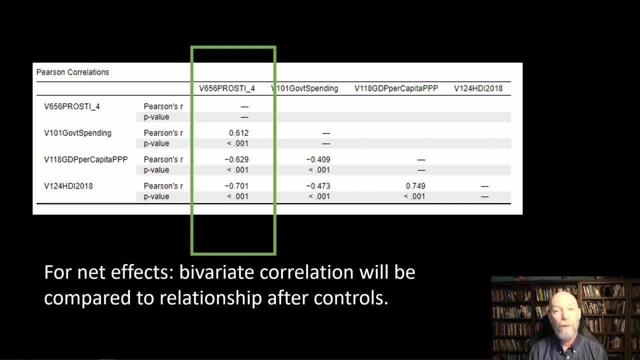 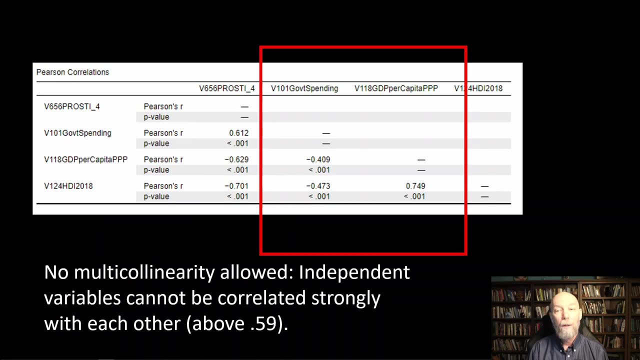 Strong negative relationship. Both the government spending and prostitution view and the HDI and prostitution view results are strong, So we're going to have to look at that Now. we've never used this other side of the correlation matrix, but these values tell us how each 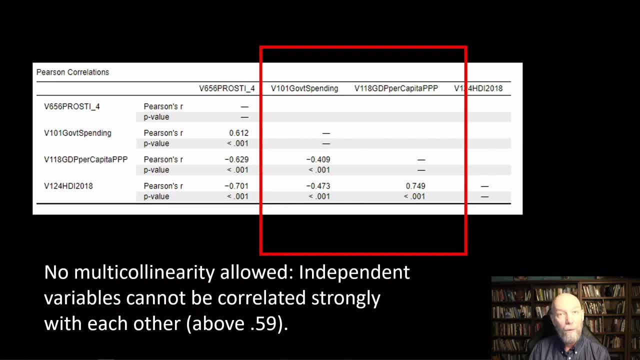 independent variable relates to the other independent variables And, as I said before, no multicollinearity is saying that we cannot have any two independent variables strongly related to each other. So we need to make sure that none of these variables are correlated beyond, say, 0.59.. So if I have a 0.6 or higher, then I need to be concerned. So what do I have here? I have a 0.409.. It doesn't matter the sign- Negative or positive- is direction of effect. We're just looking at strength of relationship here. 0.409, no problem. 0.473, no problem, Oh, 0.749.. Too much, Too much correlation between these two variables. 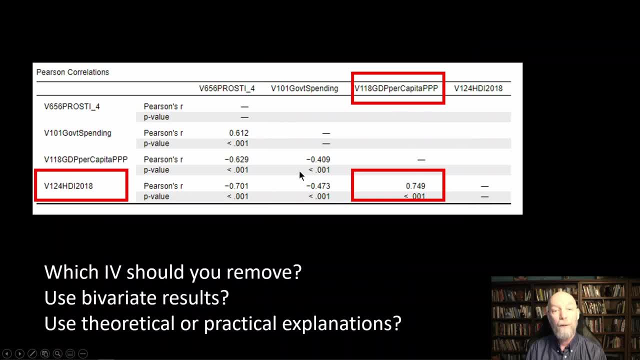 Between GDP per capita and HDI. Now, this isn't terribly surprising because HDI has a measure of average income And average income and consumption and all those things are tied to the GDP per capita right. Income levels and consumption are basically related in a larger economy, So we're not shocked to find these related. but that's a problem because it means that these two things are related. 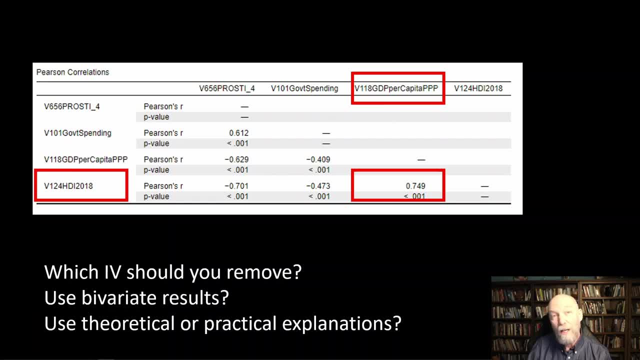 are, to a certain extent, measuring some of the same economic realities, So one of them has to go. Which one should we remove? You could, if you wish you could, look at the bivariate results and you could say: well, I want to keep in the stronger of the two. when I looked at the bivariate results, So when I tried to find out how they were related with the view of prostitution, I saw that GDP per capita had a 0.62 strength and HDI had a 0.62 strength. 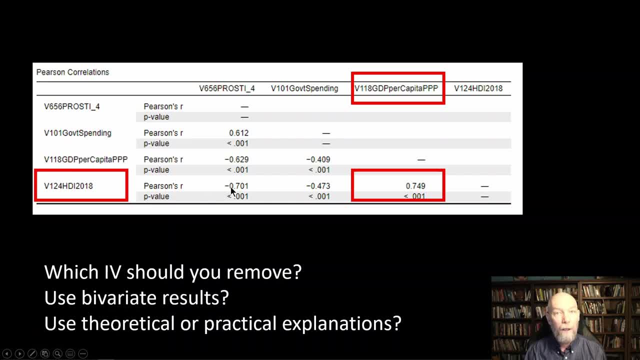 0.71.. And I might say: well, I'm going to keep 0.701 because I want to keep my best predictors in this model. That's legitimate. You could do that You also, and maybe you really should think about theoretical or practical understandings of how these things might be related and which ones matter. So I might say to myself: if I'm trying to explain the percent of the population that says prostitution is never justifiable, do I want a measure of their basic income? 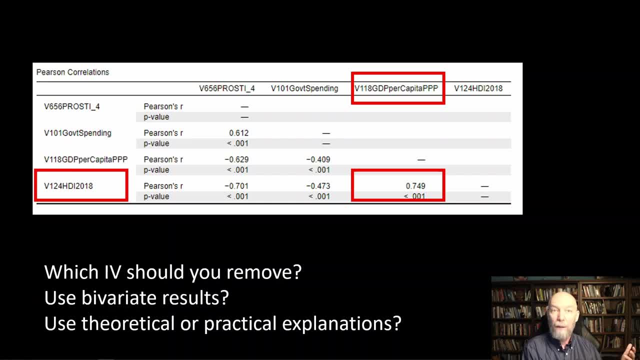 Do I want a measure of their basic GDP as something that I theoretically believe is related to cultural views of prostitution, Or do I think that a measure that collectively looks at education levels, looks at income levels and looks at life expectancy might be more important for why I think prostitution views change, And if you unpack your own explanation for what you think matters, then you may decide to keep one or the other instead. 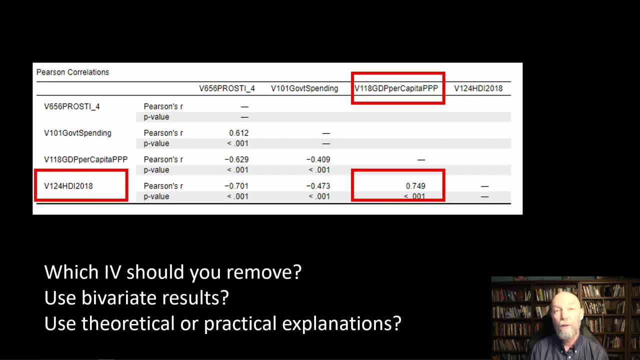 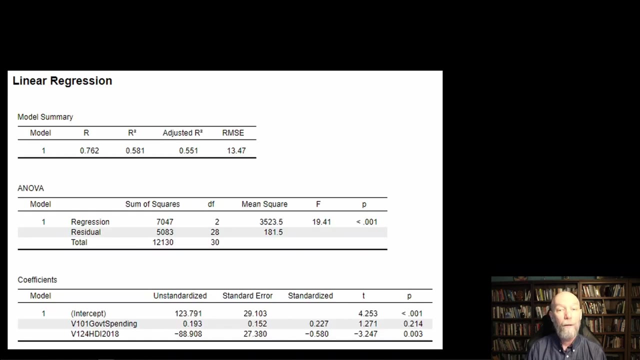 0.71.. And I might say to myself, if I'm trying to explain the percent of the population that says prostitution is never justifiable, do I want a measure of their basic income Or do I think prostitution? views change And if you unpack your own explanation for what you think matters, then you may decide to keep one or the other instead. 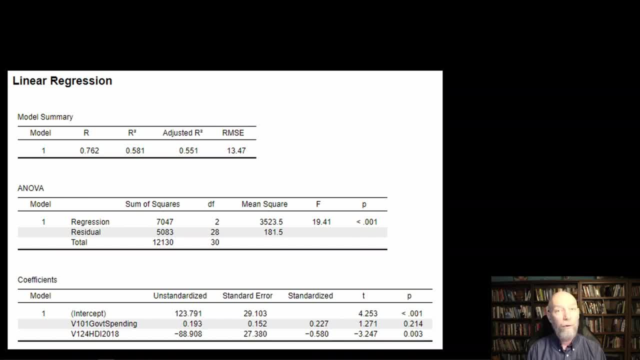 0.71.. And I might say to myself, if I'm trying to explain the percent of the population that says prostitution is never justifiable, do I want a measure of their basic income Or do I think prostitution? views change And if you unpack your own explanation for what you think matters, then you may decide to keep one or the other instead. 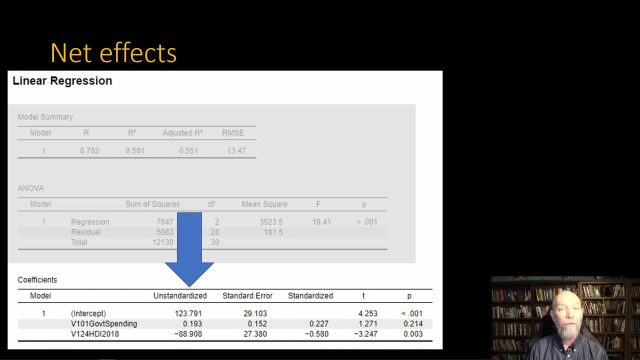 0.71.. And I might say to myself, if I'm trying to explain the percent of the population that says prostitution is never justifiable, do I want a measure of their basic income Or do I think prostitution? views change And if you unpack your own explanation for what you think matters, then you may decide to keep one or the other instead. 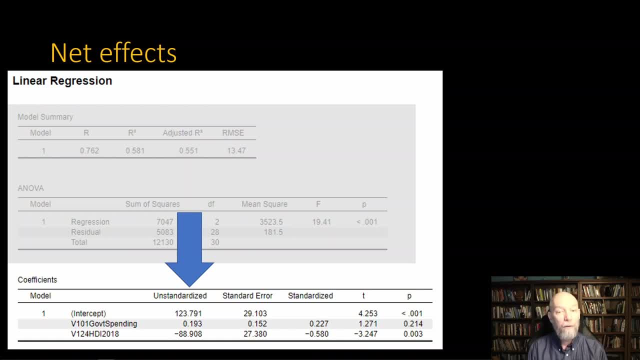 0.71.. And I might say to myself, if I'm trying to explain the percent of the population that says prostitution is never justifiable, do I want a measure of their basic income Or do I think prostitution? views change And if you unpack your own explanation for what you think matters, then you may decide to keep one or the other instead. 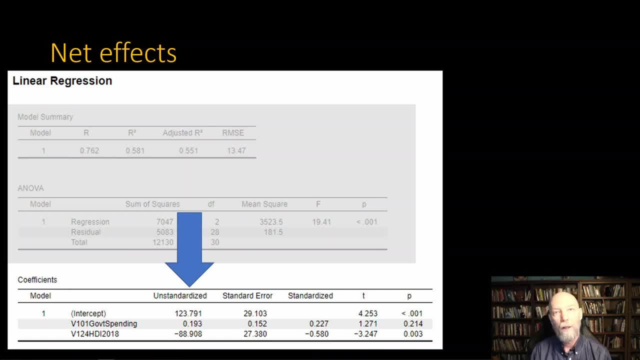 0.71.. And I might say to myself, if I'm trying to explain the percent of the population that says prostitution is never justifiable, do I want a measure of their basic income Or do I think prostitution? views change And if you unpack your own explanation for what you think matters, then you may decide to keep one or the other instead. 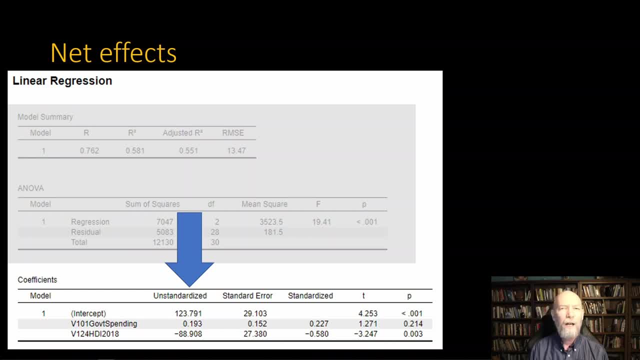 0.71.. And I might say to myself, if I'm trying to explain the percent of the population that says prostitution is never justifiable, do I want a measure of their basic income Or do I think prostitution? views change And if you unpack your own explanation for what you think matters, then you may decide to keep one or the other instead. 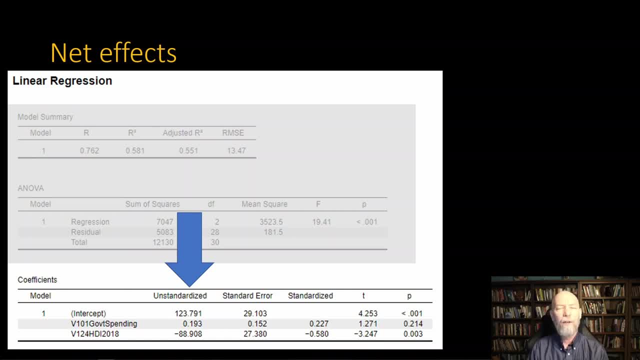 0.71.. And I might say to myself, if I'm trying to explain the percent of the population that says prostitution is never justifiable, do I want a measure of their basic income Or do I think prostitution? views change And if you unpack your own explanation for what you think matters, then you may decide to keep one or the other instead. 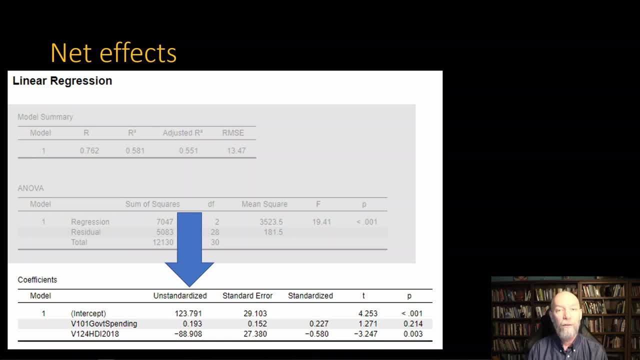 0.71.. And I might say to myself, if I'm trying to explain the percent of the population that says prostitution is never justifiable, do I want a measure of their basic income Or do I think prostitution? views change And if you unpack your own explanation for what you think matters, then you may decide to keep one or the other instead. 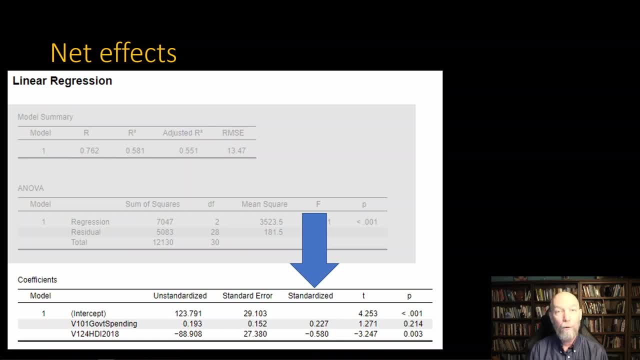 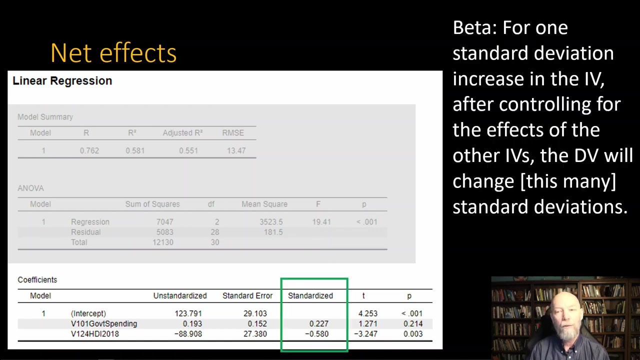 0.71.. And I might say to myself, if I'm trying to explain the percent of the population that says prostitution is never justifiable, do I want a measure of their basic income Or do I think prostitution? views change And if you unpack your own explanation for what you think matters, then you may decide to keep one or the other instead. 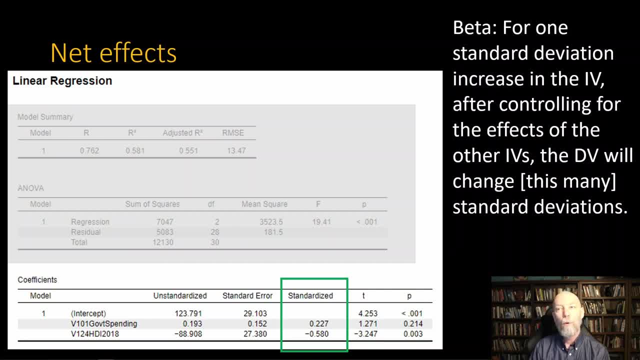 0.71.. And I might say to myself, if I'm trying to explain the percent of the population that says prostitution is never justifiable, do I want a measure of their basic income Or do I think prostitution? views change And if you unpack your own explanation for what you think matters, then you may decide to keep one or the other instead. 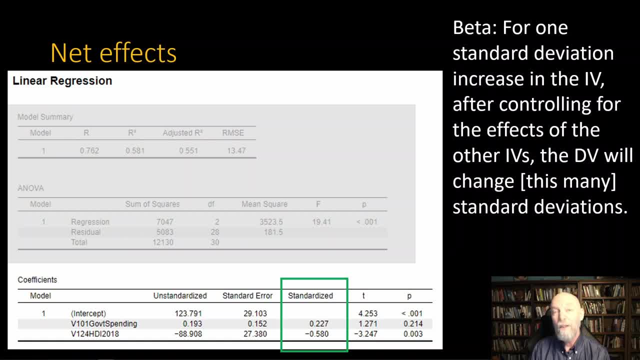 0.71.. And I might say to myself, if I'm trying to explain the percent of the population that says prostitution is never justifiable, do I want a measure of their basic income Or do I think prostitution? views change And if you unpack your own explanation for what you think matters, then you may decide to keep one or the other instead. 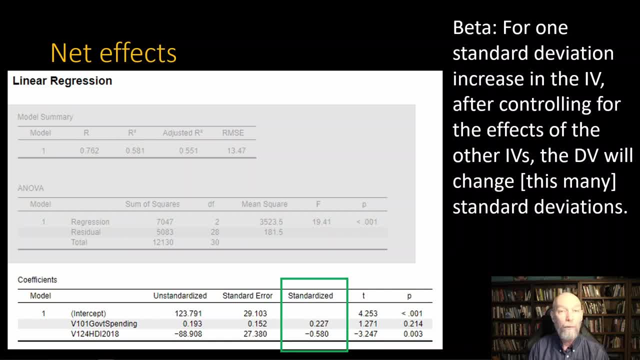 0.71.. And I might say to myself, if I'm trying to explain the percent of the population that says prostitution is never justifiable, do I want a measure of their basic income Or do I think prostitution? views change And if you unpack your own explanation for what you think matters, then you may decide to keep one or the other instead. 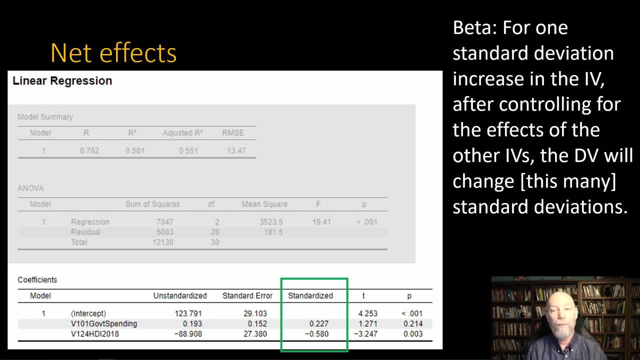 0.71.. And I might say to myself, if I'm trying to explain the percent of the population that says prostitution is never justifiable, do I want a measure of their basic income Or do I think prostitution? views change And if you unpack your own explanation for what you think matters, then you may decide to keep one or the other instead. 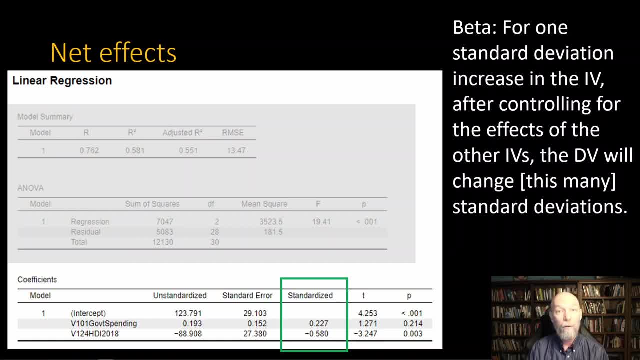 0.72.. And I might say to myself, if I'm trying to explain the percent of the population that says prostitution is never justifiable, do I want a measure of their basic income Or do I think prostitution? views change And if you unpack your own explanation for what you think matters, then you may decide to keep one or the other instead. 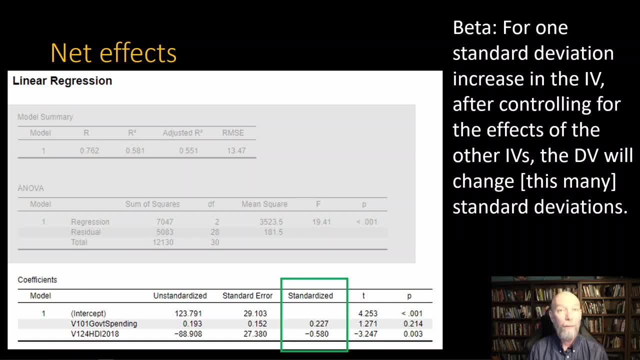 0.73.. And I might say to myself, if I'm trying to explain the percent of the population that says prostitution is never justifiable, do I want a measure of their basic income Or do I think prostitution? views change And if you unpack your own explanation for what you think matters, then you may decide to keep one or the other instead. 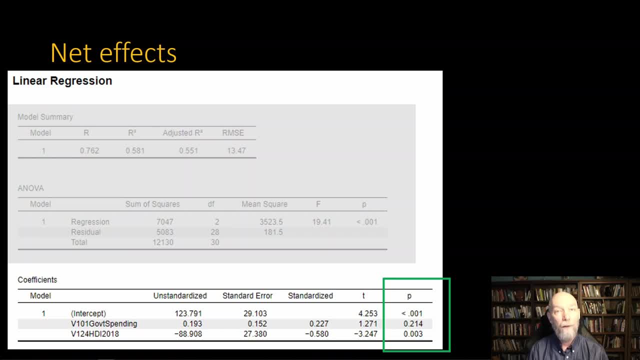 0.72.. And I might say to myself, if I'm trying to explain the percent of the population that says prostitution is never justifiable, do I want a measure of their basic income Or do I think prostitution? views change And if you unpack your own explanation for what you think matters, then you may decide to keep one or the other instead. 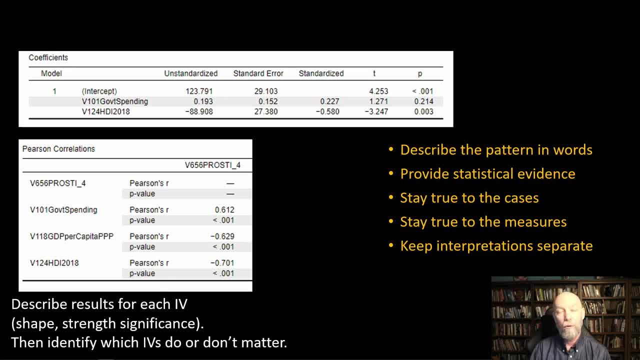 0.73.. And I might say to myself, if I'm trying to explain the percent of the population that says prostitution is never justifiable, do I want a measure of their basic income Or do I think prostitution? views change And if you unpack your own explanation for what you think matters, then you may decide to keep one or the other instead. 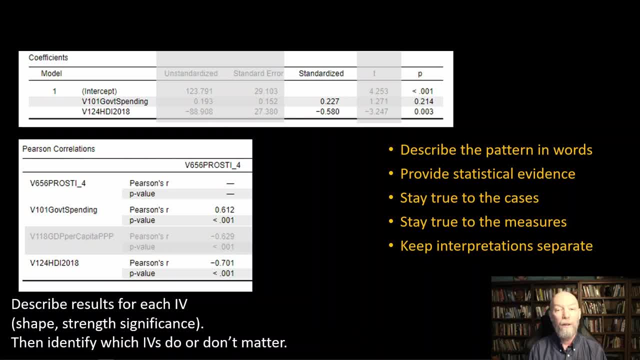 0.72.. And I might say to myself, if I'm trying to explain the percent of the population that says prostitution is never justifiable, do I want a measure of their basic income Or do I think prostitution? views change And if you unpack your own explanation for what you think matters, then you may decide to keep one or the other instead. 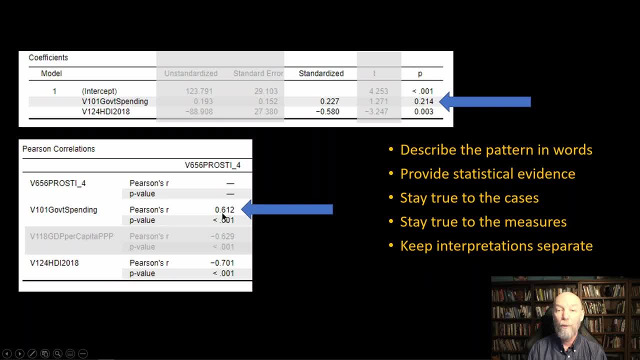 0.73.. And I might say to myself, if I'm trying to explain the percent of the population that says prostitution is never justifiable, do I want a measure of their basic income Or do I think prostitution? views change And if you unpack your own explanation for what you think matters, then you may decide to keep one or the other instead. 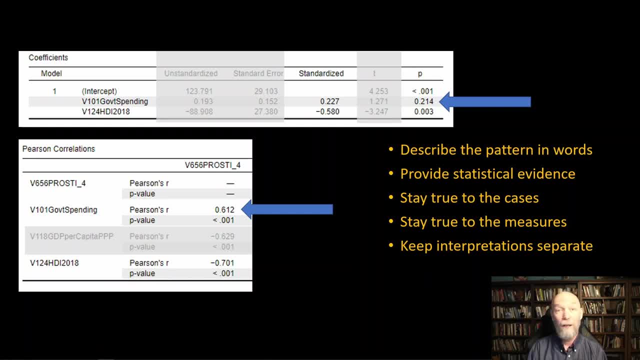 0.74.. And I might say to myself, if I'm trying to explain the percent of the population that says prostitution is never justifiable, do I want a measure of their basic income Or do I think prostitution? views change And if you unpack your own explanation for what you think matters, then you may decide to keep one or the other instead. 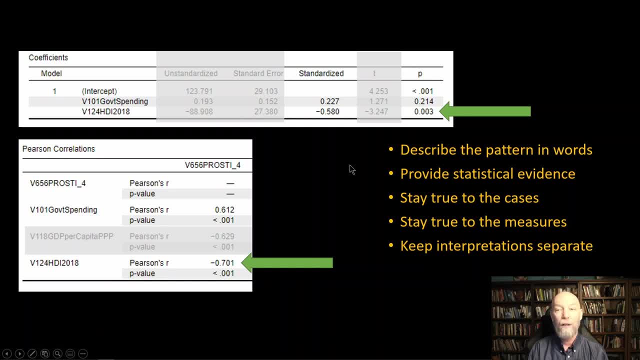 0.74.. And I might say to myself, if I'm trying to explain the percent of the population that says prostitution is never justifiable, do I want a measure of their basic income Or do I think prostitution? views change And if you unpack your own explanation for what you think matters, then you may decide to keep one or the other instead. 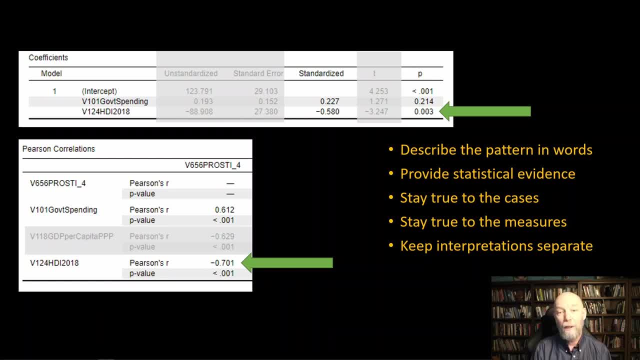 0.74.. And I might say to myself, if I'm trying to explain the percent of the population that says prostitution is never justifiable, do I want a measure of their basic income Or do I think prostitution? views change And if you unpack your own explanation for what you think matters, then you may decide to keep one or the other instead. 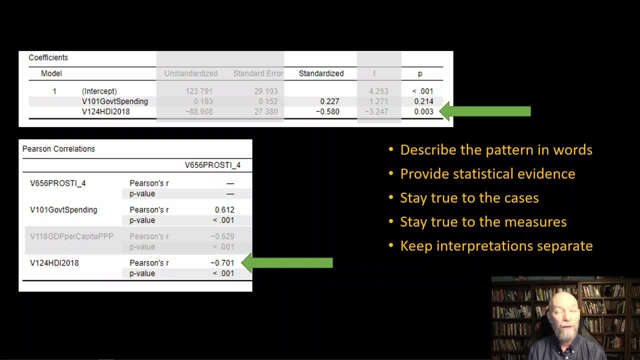 0.74.. And I might say to myself, if I'm trying to explain the percent of the population that says prostitution is never justifiable, do I want a measure of their basic income Or do I think prostitution? views change And if you unpack your own explanation for what you think matters, then you may decide to keep one or the other instead. 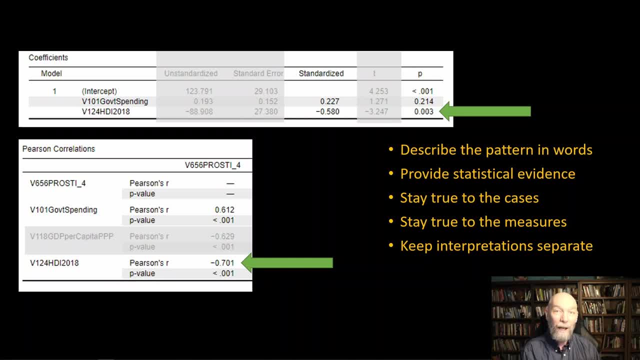 0.74.. And I might say to myself, if I'm trying to explain the percent of the population that says prostitution is never justifiable, do I want a measure of their basic income Or do I think prostitution? views change And if you unpack your own explanation for what you think matters, then you may decide to keep one or the other instead. 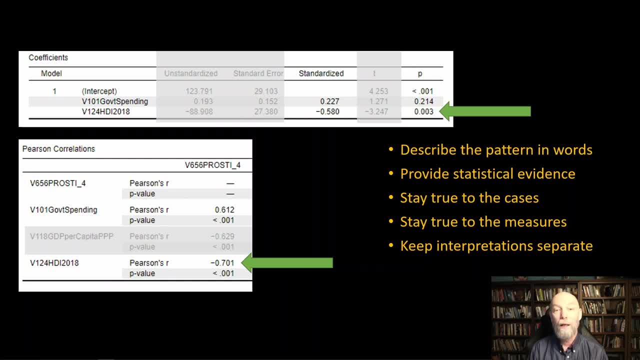 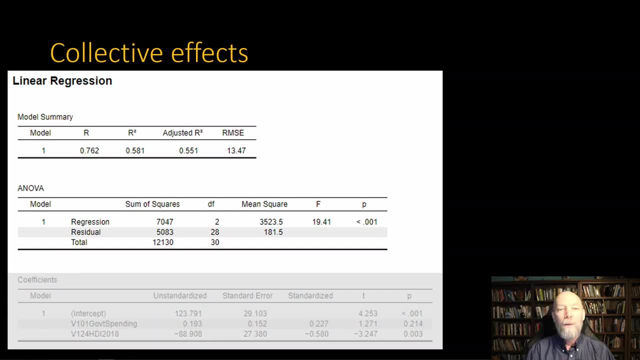 0.74.. And I might say to myself, if I'm trying to explain the percent of the population that says prostitution is never justifiable, do I want a measure of their basic income Or do I think prostitution? views change And if you unpack your own explanation for what you think matters, then you may decide to keep one or the other instead. 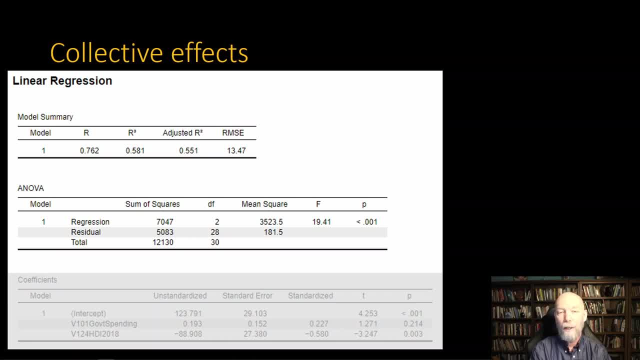 0.74.. And I might say to myself, if I'm trying to explain the percent of the population that says prostitution is never justifiable, do I want a measure of their basic income Or do I think prostitution? views change And if you unpack your own explanation for what you think matters, then you may decide to keep one or the other instead. 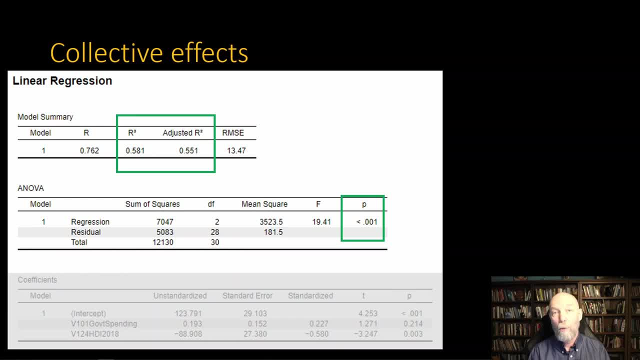 0.74.. And I might say to myself, if I'm trying to explain the percent of the population that says prostitution is never justifiable, do I want a measure of their basic income Or do I think prostitution? views change And if you unpack your own explanation for what you think matters, then you may decide to keep one or the other instead. 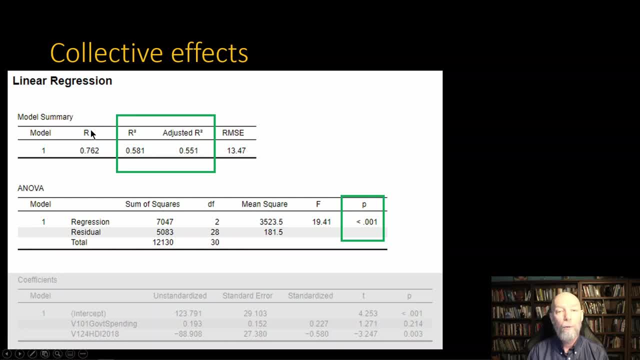 0.74.. And I might say to myself, if I'm trying to explain the percent of the population that says prostitution is never justifiable, do I want a measure of their basic income Or do I think prostitution? views change And if you unpack your own explanation for what you think matters, then you may decide to keep one or the other instead. 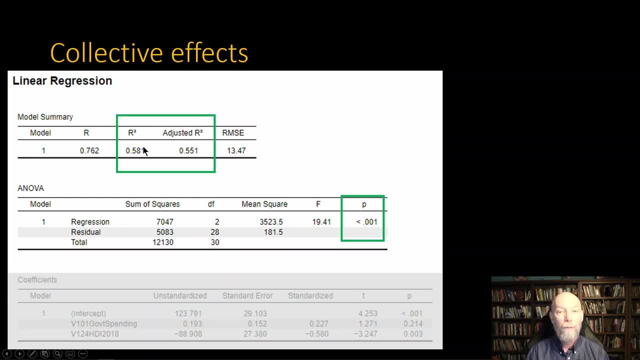 0.74.. And I might say to myself, if I'm trying to explain the percent of the population that says prostitution is never justifiable, do I want a measure of their basic income Or do I think prostitution? views change And if you unpack your own explanation for what you think matters, then you may decide to keep one or the other instead. 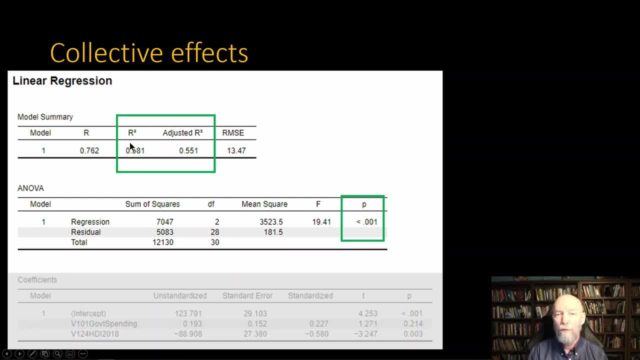 0.74.. And I might say to myself, if I'm trying to explain the percent of the population that says prostitution is never justifiable, do I want a measure of their basic income Or do I think prostitution? views change And if you unpack your own explanation for what you think matters, then you may decide to keep one or the other instead. 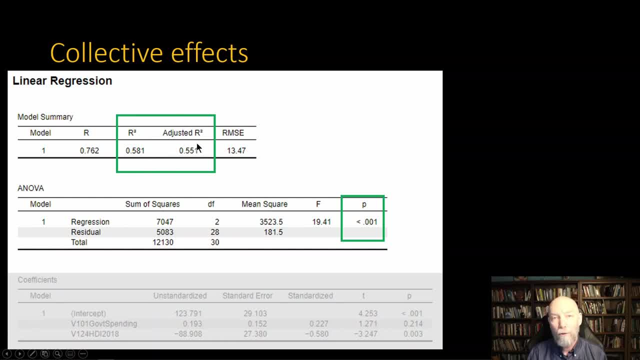 0.74.. And I might say to myself, if I'm trying to explain the percent of the population that says prostitution is never justifiable, do I want a measure of their basic income Or do I think prostitution? views change And if you unpack your own explanation for what you think matters, then you may decide to keep one or the other instead. 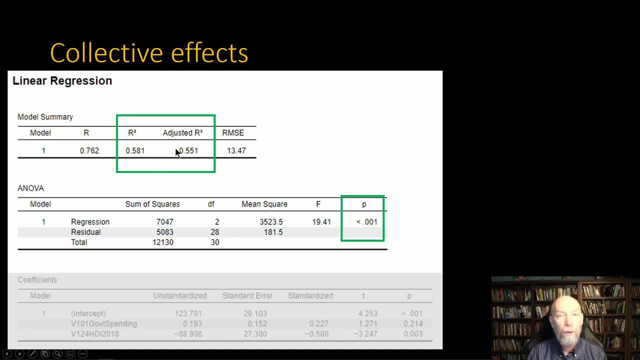 0.74.. And I might say to myself, if I'm trying to explain the percent of the population that says prostitution is never justifiable, do I want a measure of their basic income Or do I think prostitution? views change And if you unpack your own explanation for what you think matters, then you may decide to keep one or the other instead. 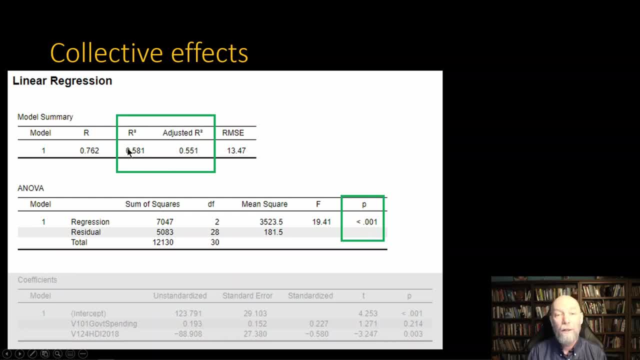 0.74.. And I might say to myself, if I'm trying to explain the percent of the population that says prostitution is never justifiable, do I want a measure of their basic income Or do I think prostitution? views change And if you unpack your own explanation for what you think matters, then you may decide to keep one or the other instead. 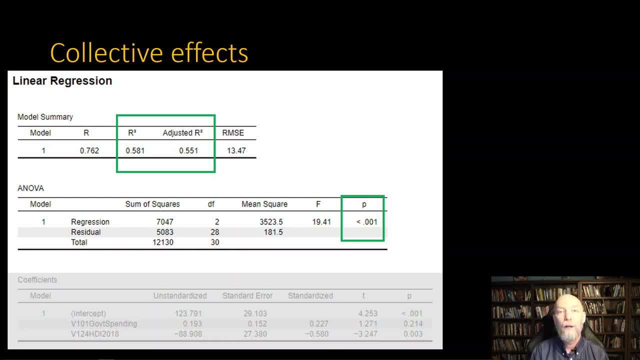 0.74.. And I might say to myself, if I'm trying to explain the percent of the population that says prostitution is never justifiable, do I want a measure of their basic income Or do I think prostitution? views change And if you unpack your own explanation for what you think matters, then you may decide to keep one or the other instead.